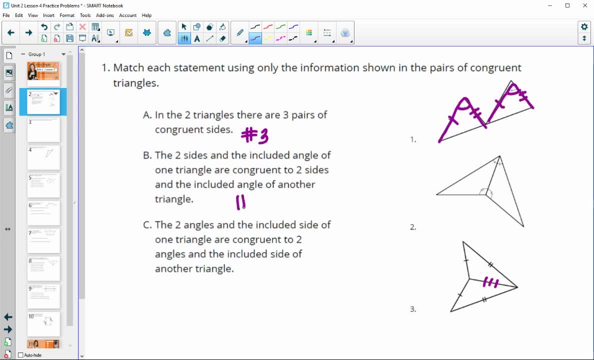 and the included angle of another. So B is number one. And then C says that it's two angles and the included side of one. Okay, So we've got two angles here and the included side would be this side. that's the same in both, And then two angles. 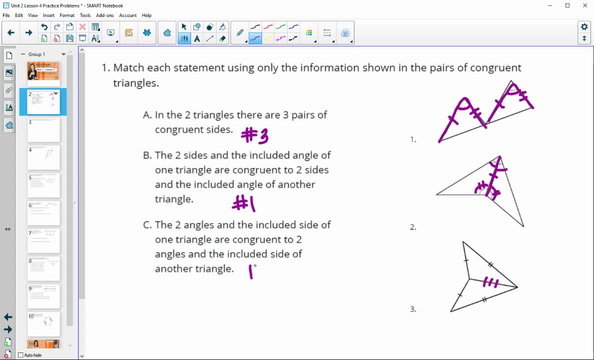 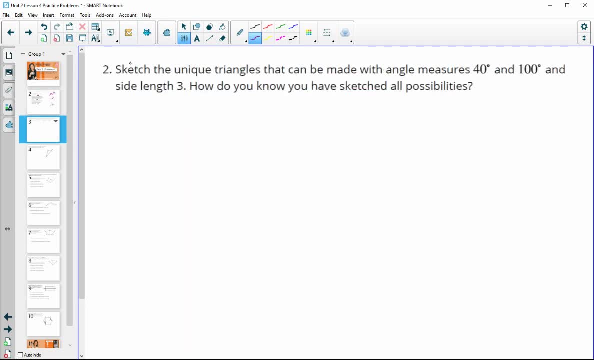 and the included side of another. So C is number two. Number two sketch the unique triangles that can be made with angle measures of 40 and 100 degrees and a side length of three. So let me get a ruler here and we'll do a side length of three inches. 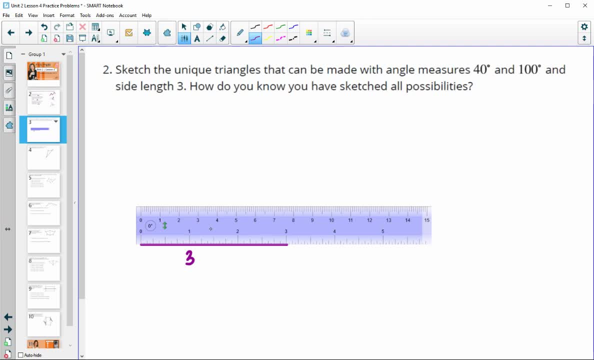 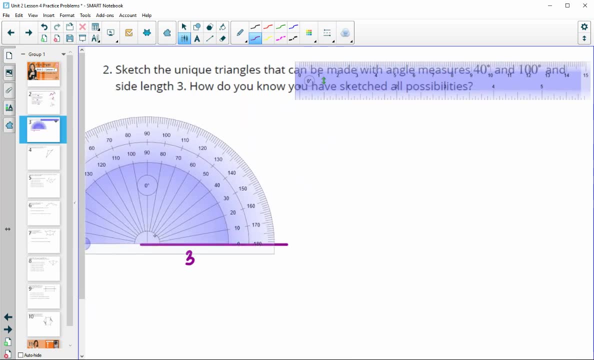 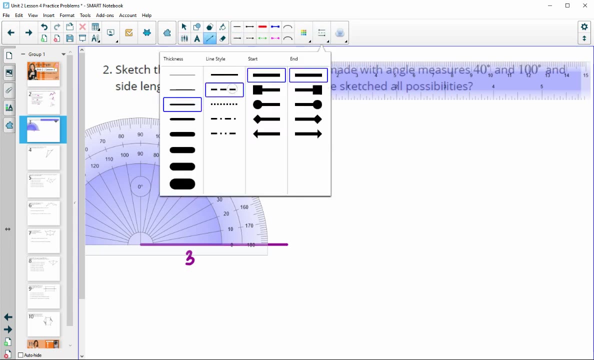 So we could know that this side here is three, And then we could do the protractor and do a 40 degree angle from this side. Okay, So here's 40. And so if I just let me do a dotted line here, since we don't know where this is going to end, 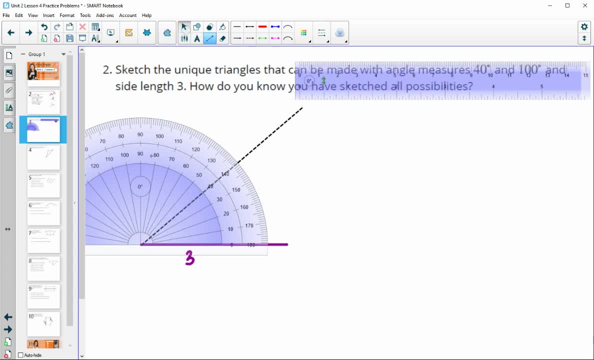 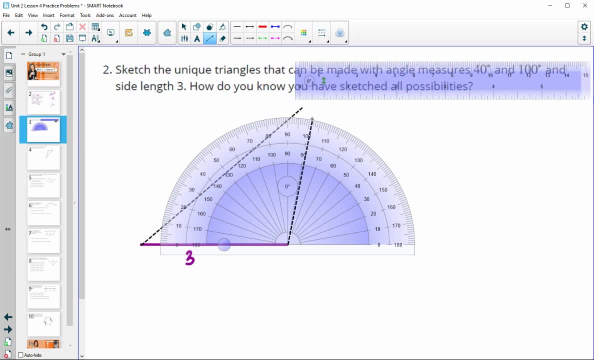 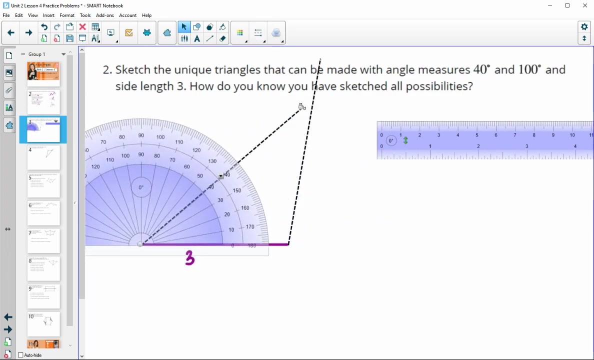 So this would be a 40 degree angle, And then we could do the 100 degree angle from this side And so from this side go to a 100 degree angle, and then we would just extend these Until they crossed, And that would make us our triangle. So let me just move this So I can extend this 40 degree angle. 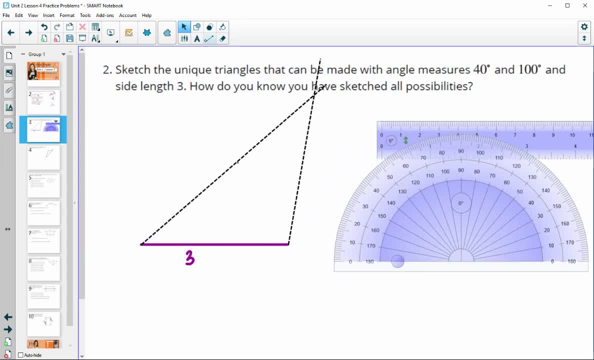 And then that would create one of the triangles. Oops, So then we would have this triangle here And that would have A three unit side. here We did the 40 degree angle here. This one is 100 degrees And we know a triangle total is 180. So if we subtract those from 180, we also get 40 degrees for this one. 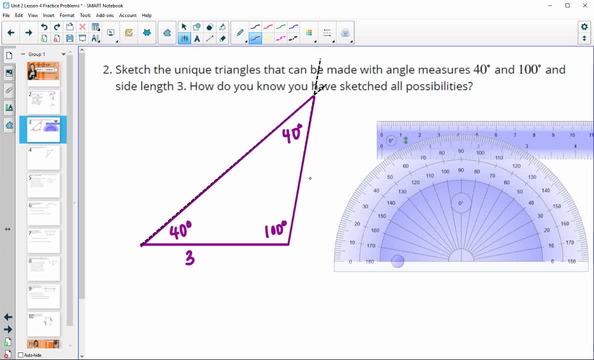 But there's one of the triangles, And then by isosceles we would know that this one is also three, So both of these sides ended up being the same. So that's one of the triangles that could be created. 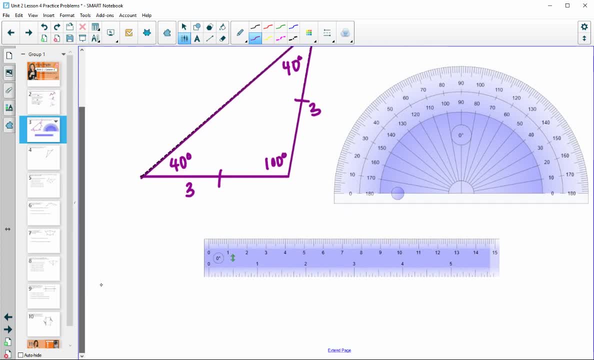 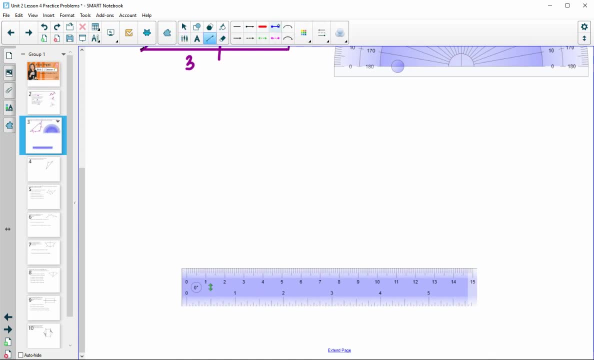 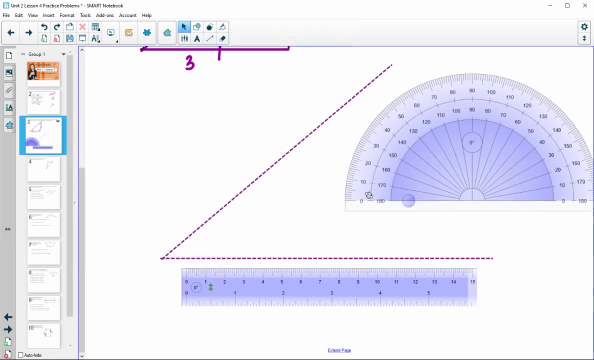 We could also have That 40 degree angle, And let me just kind of start with a dotted line side here, And then we could do The 40 degree angle from here. So there's a 40 degree angle And then we could actually measure. 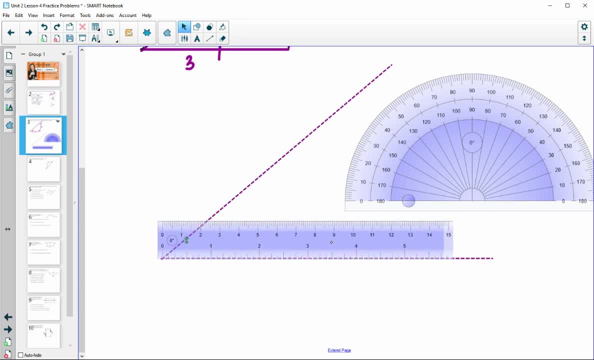 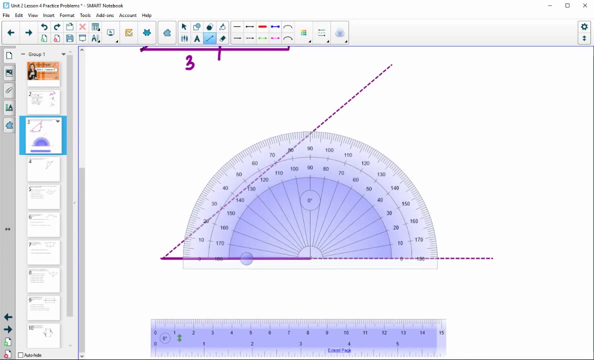 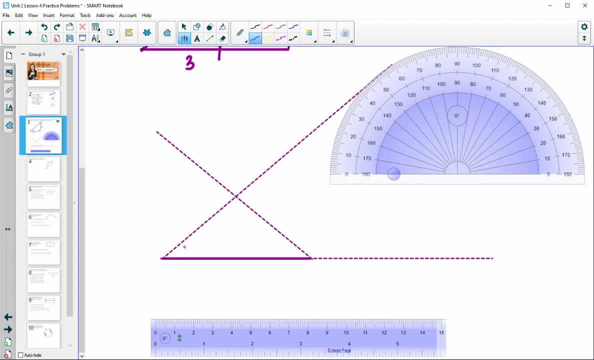 Um, The three here. So I'm going to measure that three here, And then we could do another 40 degree angle from this side. Instead of the 100 degree angle we could do a 40 degree angle here, And then that would create a new triangle as well. 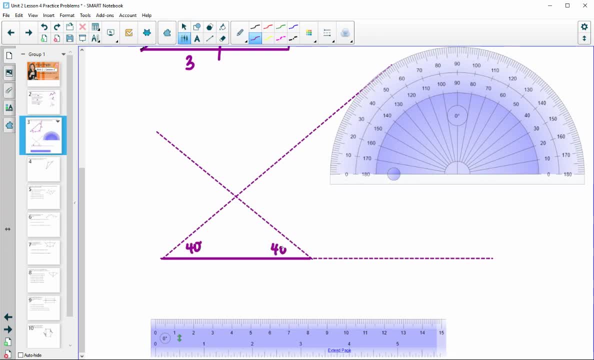 So this would be: We did 40 here, And we did another 40 here, So that this one would be the 100.. And then this would be the three, And so there's Another unique triangle that could have been. 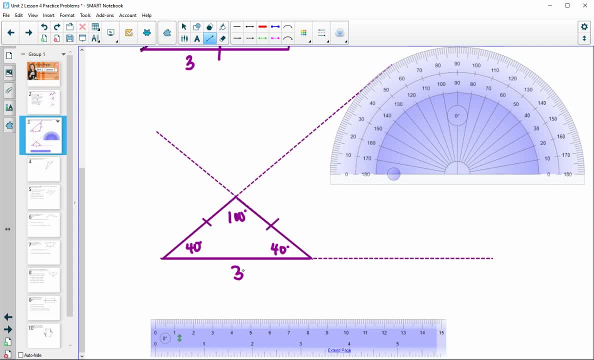 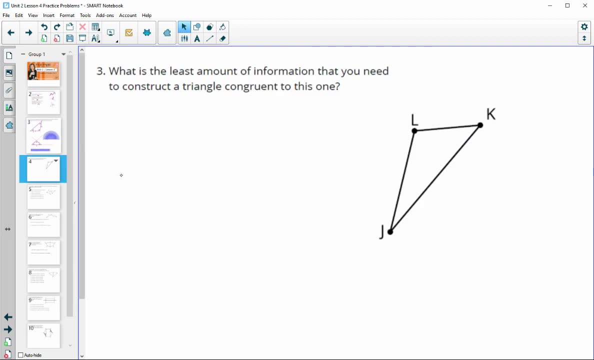 Drawn, Where these sides are the same length but they're not three. And then that bottom one, The longest one, is three, Number three. What's the least amount of information you would need to construct this triangle. Now, there's going to be. You could pick different parts. 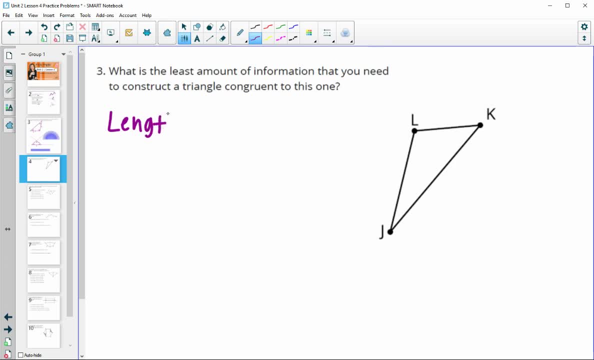 Um, But you're going to need to know the length Of a side. So I'm going to say the length, If I knew the length of LK, And then I knew the measure Of two of the angles, So I'm just going to say the measure of angle L. 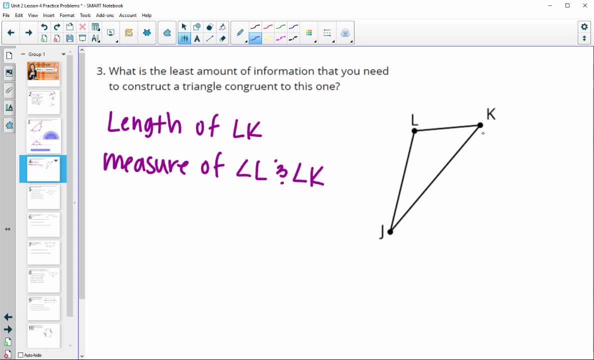 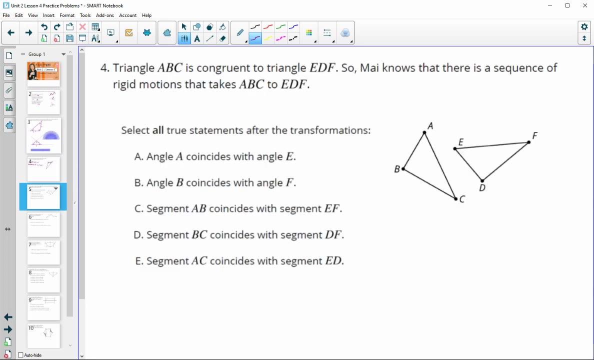 And the measure of angle K. So I know this side length And then I would know this angle measure And this angle measure, Then I would be able to create Um, The entire triangle Number four, Triangle ABC is congruent to triangle EDF. 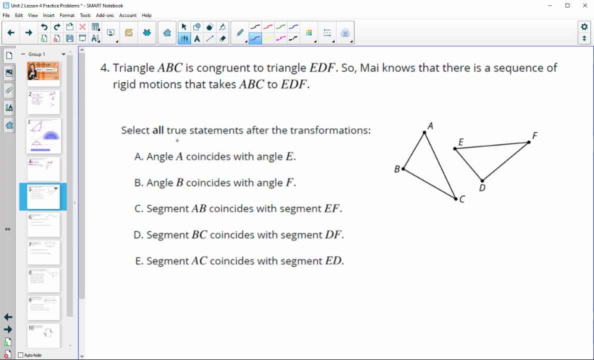 So my knows there's a sequence of rigid motions That takes one to the next. Select all true statements. A coincides with E, So A is the first letter. E is the first letter, So that is true. B coincides with F. 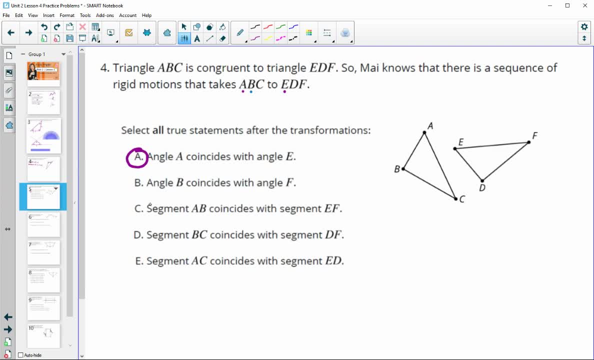 So B is the second letter, F is the third letter. So this is true. So this is false. Segment AB Coincides with segment EF. So AB are the first two letters, EF are the first and last. 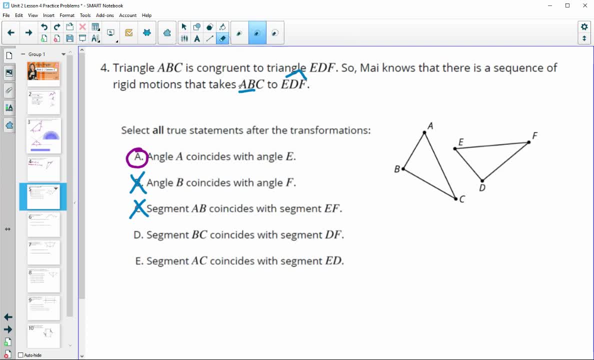 So that's going to be false. Those are not corresponding. BC Coincides with DF. So BC is the last two letters, DF are the last two letters, So that is true. Segment AC Coincides with ED. 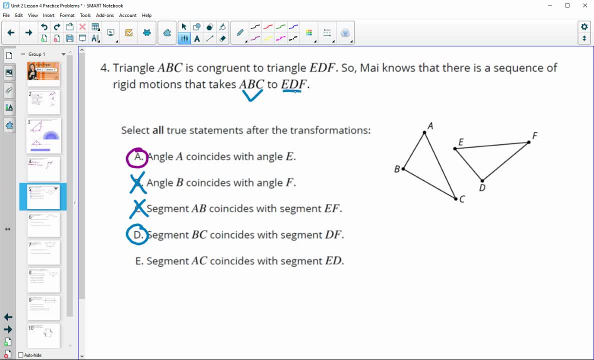 So AC is first and last, ED is first and second. So that's going to be false. Number five A: rotation by angle ACE Using point C as the center Takes CBA on to CDE. So we know rotating by this angle. 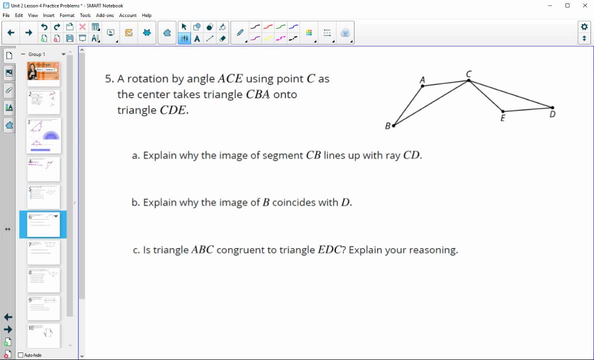 Number six, A, rotation by angle ACE Using point C, as the center Takes CBA on to CDE. So we know rotating by this angle Takes one triangle on to the next. So explain why the image of CB lines up with ray CD. 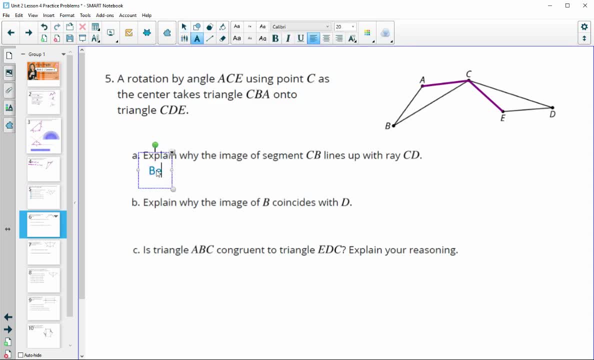 And that's because that's how we defined it. We said that the rotation by angle ACE is going to take this triangle on to this one. So we know that segment CB would land On Ray, And let me put that ray up here. 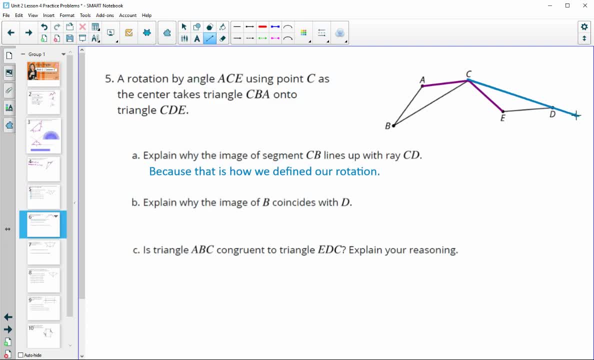 Would land on ray CD. So we know that this is going to rotate over to there. So how do we know that B will actually land? The image of B will land exactly on D, And that's because Trans Transformations- 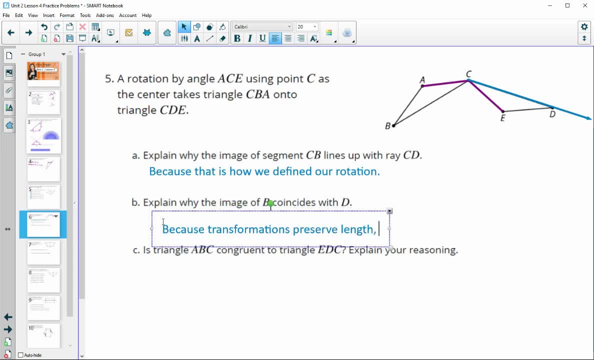 Preserve Length. So the image of B is the same distance from C as D is. So B prime or the image of B, will land exactly on D. So we knew that these two triangles were congruent. So the length of CB is going to stay the same. 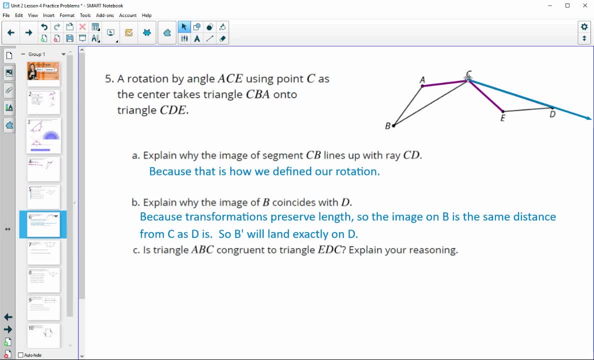 So CB, prime, B prime is the same distance from C as D is, So it's going to land in the same spot. So is triangle ABC congruent to EDC? And yes, because. so which one did we line up? We already lined up B would be on D. 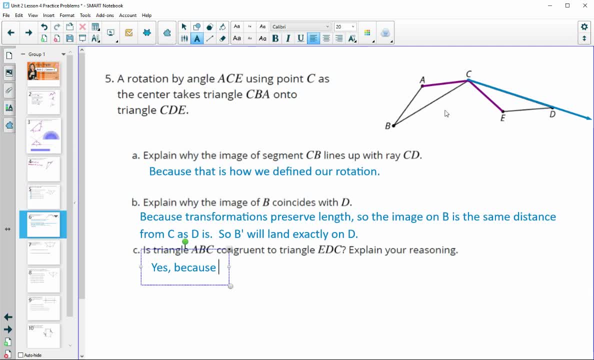 So A is also going to land on E. okay, Because the rotation will have A coincide with E. We already justified B. So B coinciding with D and C stays in the same spot. So all vertices coincide, So the two. so there is a rigid motion that takes one to the next. 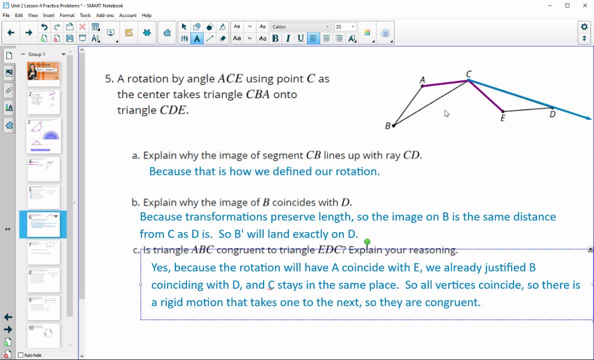 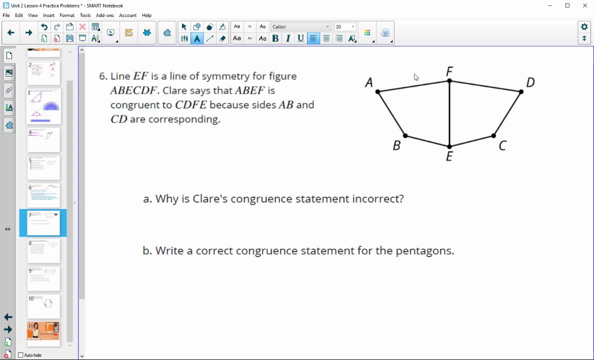 So they are congruent, All right. number six, line EF, is the line of symmetry of these two shapes. Claire says that ABEF is congruent to CDFE because AB and CD are corresponding. Why is her congruent statement wrong? 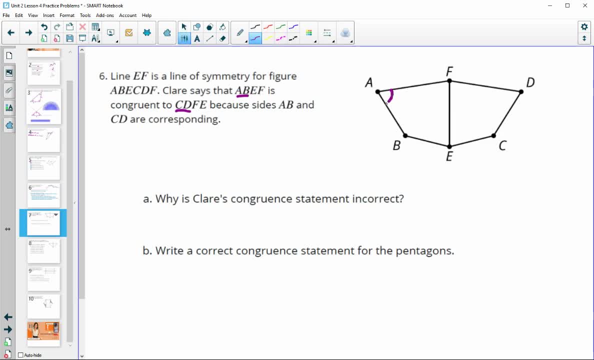 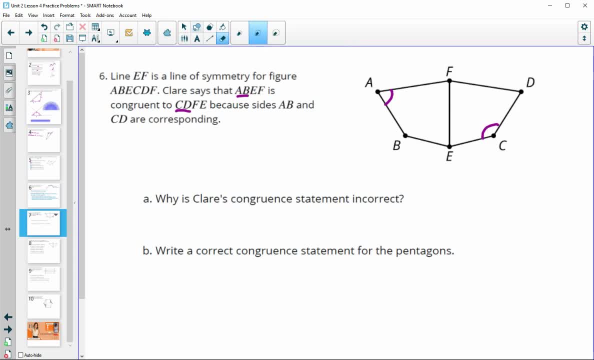 And that's incorrect because those are not corresponding angles. So we can't just match up corresponding sides, We also need to match up corresponding angles. So if we were going to write a congruent statement, that was true, so let's start with her first statement of ABEF. that would be congruent too. 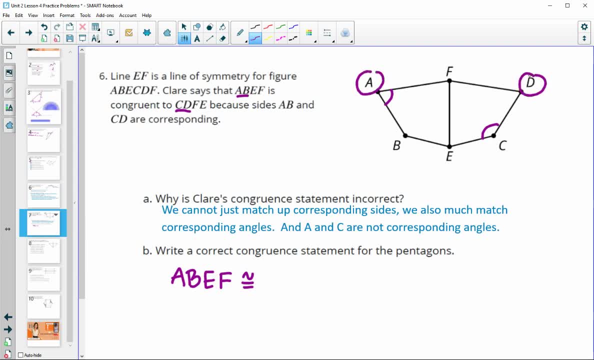 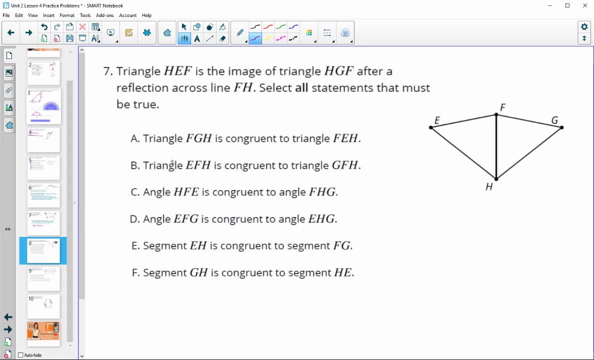 So A actually goes with D, So A actually goes with D, And then B goes with C, And then we have E with E and F with F, And then we have E with E and F with F. Number seven triangle, HEF, is the image of HGF. after a reflection. 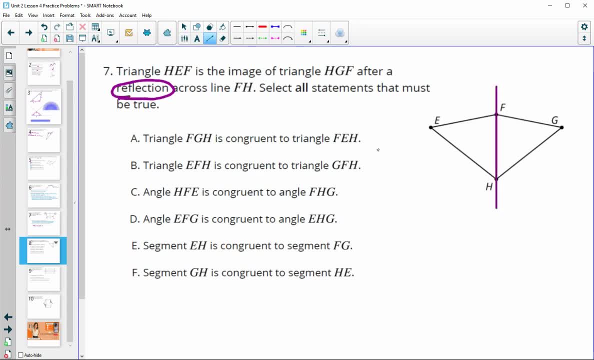 Number seven, triangle HEF, is the image of HGF. after a reflection: Okay, so we're reflecting over this line. Select all statements. that must be true. So remember: reflect means flips over, So E is going to land on G. 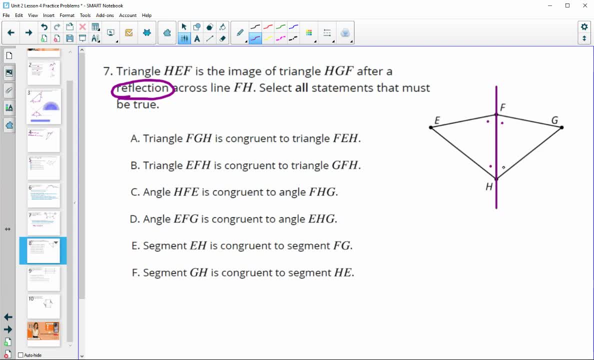 These two angles are going to be the same. They're going to flip on each other. And these two angles are going to flip on each other. So triangle F, G and F are going to flip on each other. So triangle EFH. so going like this is congruent to FEH and that is true. 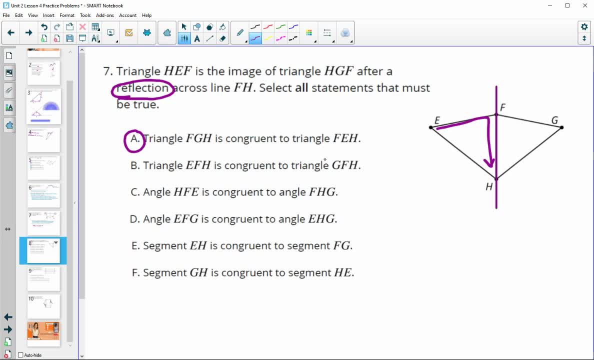 Triangle EFH is congruent to triangle GFH and that's going to match up our corresponding parts. so that's true as well. Angle HFUP. So our proof is going to be in the triangle EFH- FE. so this angle is congruent to HFE, is congruent to FHG- this one, that's false. 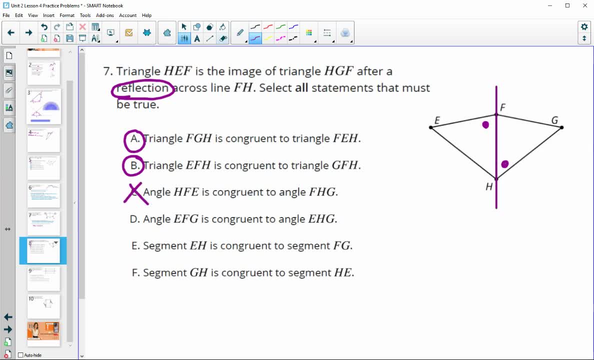 that's in a rotation that the alternating ones are the same Angle: EFG, so EFG. so this angle here is congruent to angle EHG, and that is not necessarily true in a reflection Segment EH. so this segment here is congruent to FG. that is false. And then 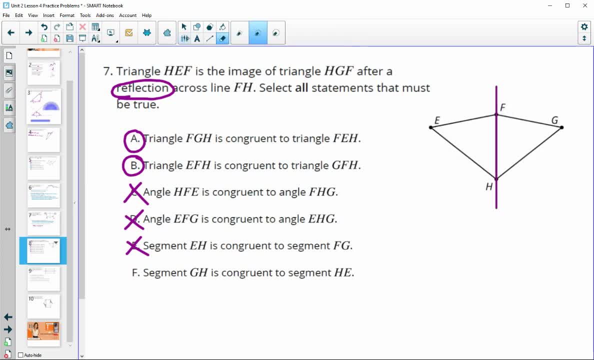 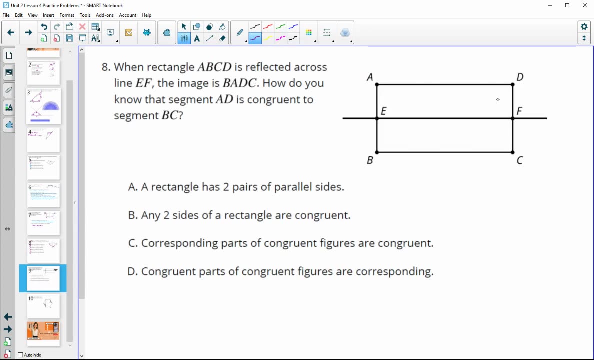 finally, Finally, segment GH is congruent to HE, and that would be true Number eight. when this rectangle ABCD is reflected across line EF, its image is BADC. So remember, these are the congruent images. They're matching up our parts. 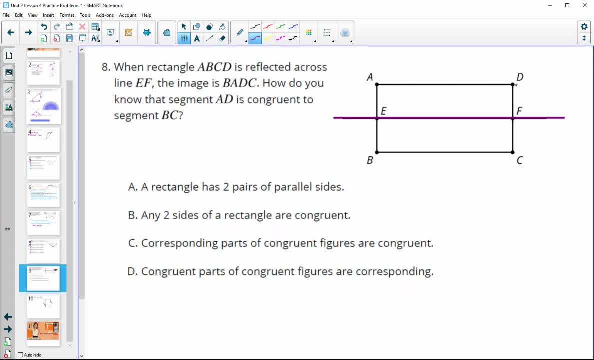 So A flips to B, B flips to A, D flips to C, C flips to D. How do we know that segment AD is congruent to BC? And so we can look here and we see that AD in the first, BC in the second.